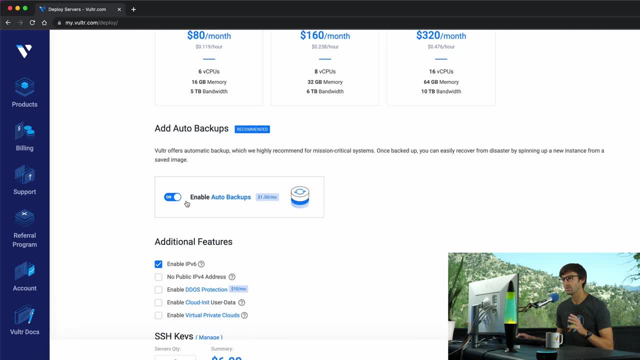 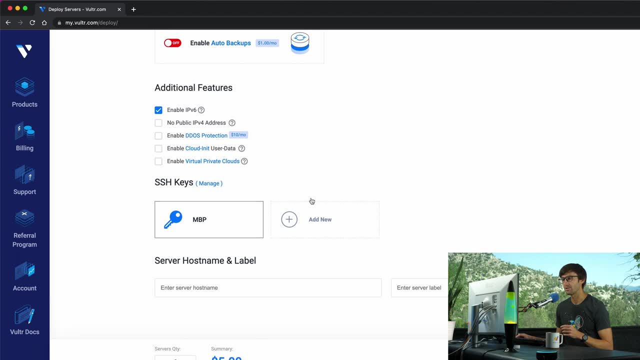 terabyte of monthly bandwidth. Okay, so we don't need any backups, unless you're again, you're doing something critical. I'm going to turn that off and everything else looks good. I do have other videos about how to set up a passwordless login with your SSH keys, but we're just going to log in with a. 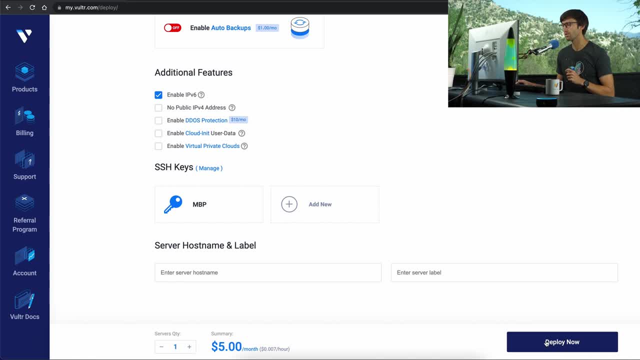 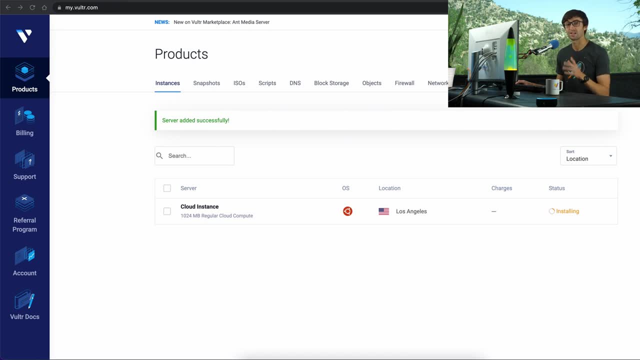 password for this and that looks good, So let's click on deploy now. This will take a little bit for this to install and get set up, so I will fast forward through this and catch up with you when that finishes. Okay, and just a few moments later, our server is up and running, as you can see here. 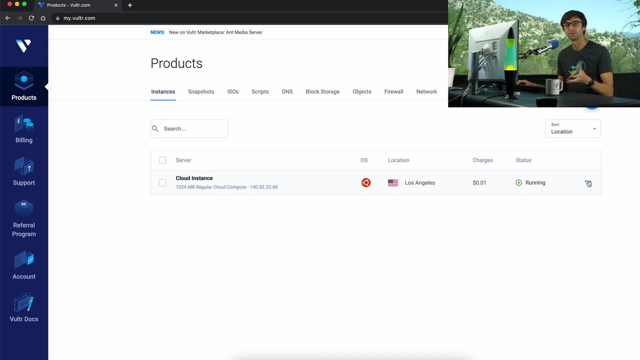 and the really cool thing about VPSs is, yes, there is a monthly rate, but you're only charged by the hour. So if I were to go right here and destroy the server right now- I'm going to be able to do that right now- I would only be charged one cent, which is really cool. So anyway, let's click. 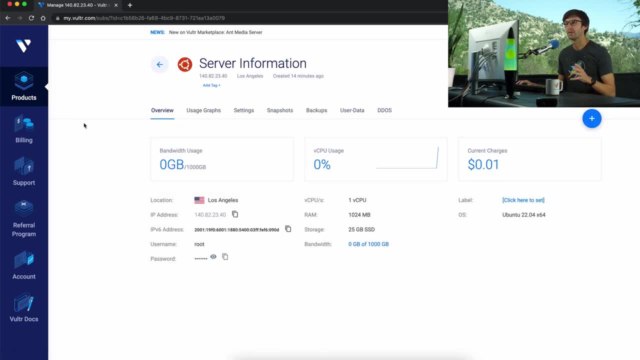 into our cloud instance and this is the page that is associated with this particular VPS. There's some good information here about our IP address, username and password. We'll be using those in just a bit. The current plan that we have selected in our operating system that's running. 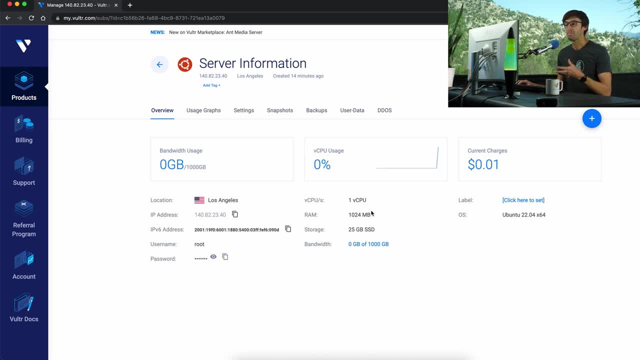 now, If we want to change any of the specs associated with our VPS, then we can do that. I'm going to show you how to do that. Also, we can change the operating system if we want to do that as well. So, in order to do that, you come into settings, change plan, and that'll allow you to increase. 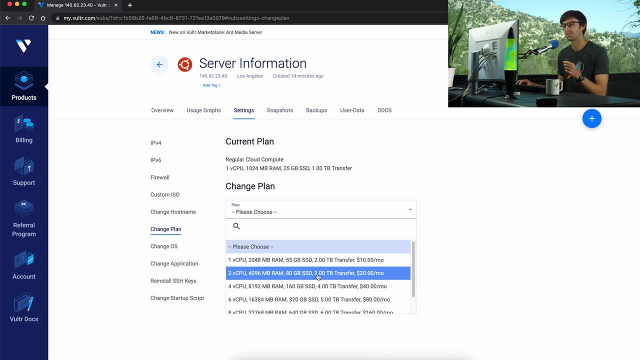 the amount of CPU cores and RAM and disk space associated with your VPS. You can also change the operating system from Ubuntu to something else or change the application that's running on top of it. We won't get into that too much, but I just want to make you aware that that. 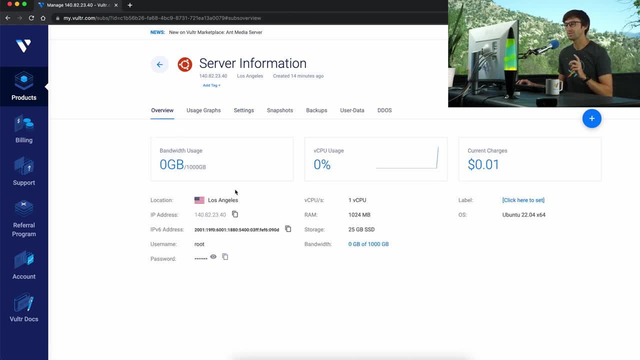 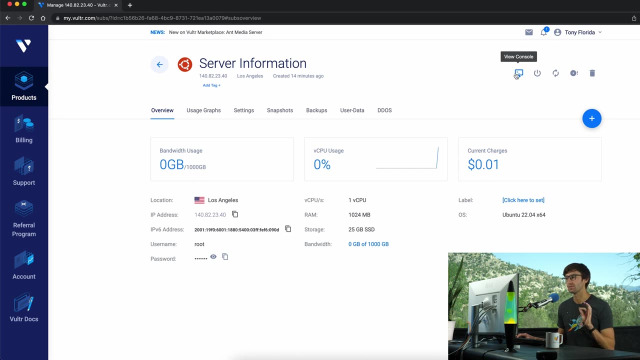 is available here. Okay, so back here, let's go ahead and log into our server. Now there's a couple different ways you can do this. You can use PuTTY on Windows. you can use a terminal on Mac or Linux. The easiest- probably for everybody- way to do this is with a built-in server console. So let's 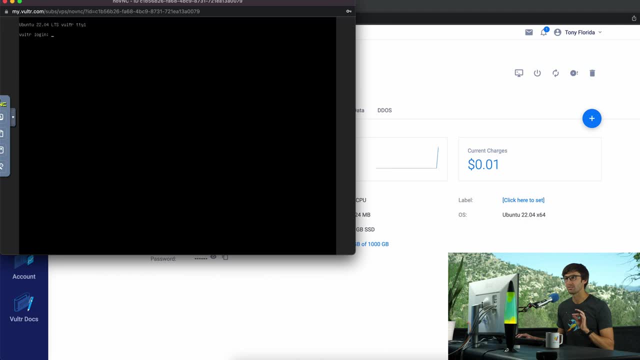 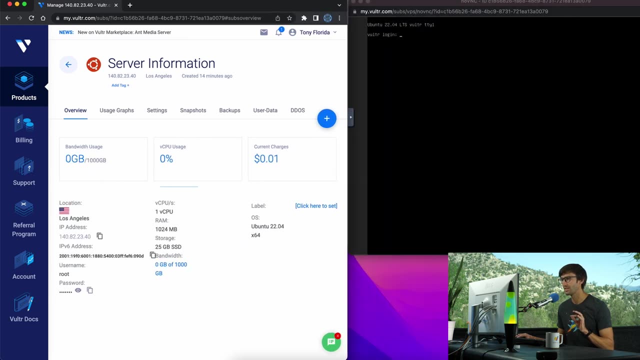 click on that and that's going to open up to something that looks like this: Vultr login. So let's put that here on the right hand side. We'll put this on the left hand side because we're going to need some information. So, Vultr login, The username is root, so go ahead and type that in. 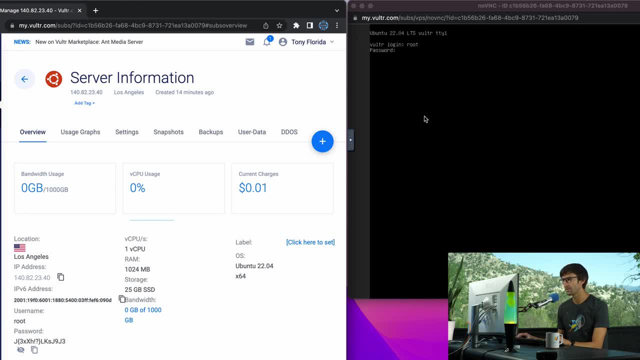 And then the password. Let's show the password here. Unfortunately, I don't think there's any way to paste into here. Oh, maybe there is, but I'm just going to type this in right now and you won't see anything happen as you type. but when you're done you can just hit enter and that'll go ahead, and 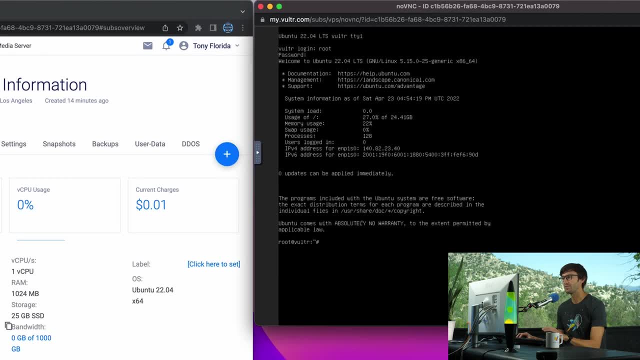 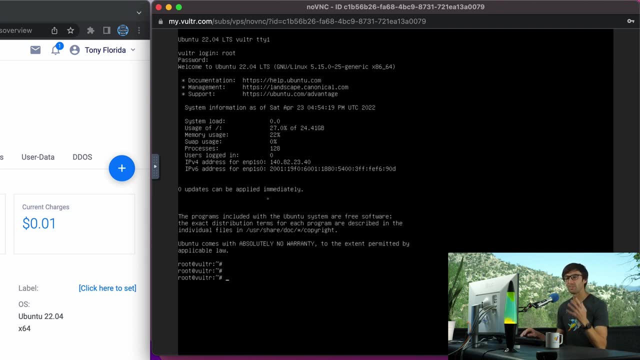 log you into your VPS Now. this, as you can see, here is an Ubuntu system. Welcome to Ubuntu 22.04. and this is the terminal command line session that we have logged ourselves into. Now it looks like it's up to date. Zero updates can be applied immediately, but it's always good practice if 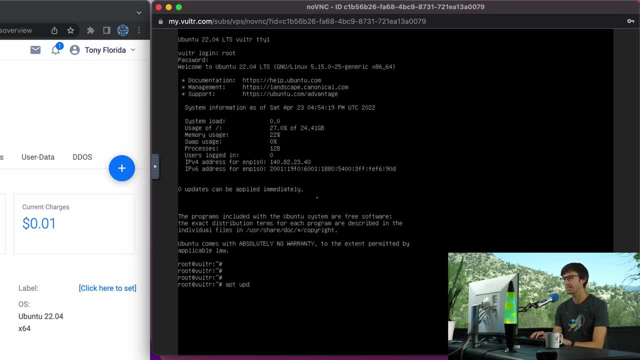 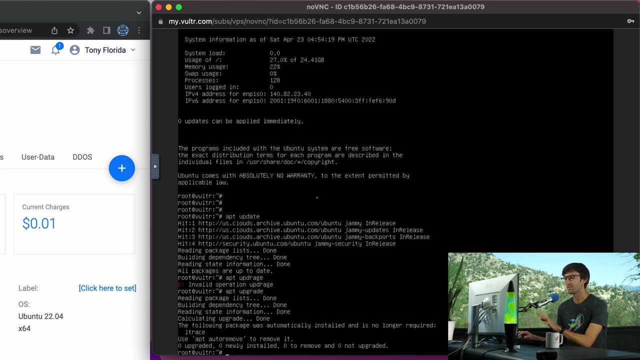 this is not the case, to do something like this apt update- And this is going to update the list of packages and you can do an apt upgrade- And because everything's already up to date, there is no updates to be applied. but again, that's just good practice to make sure your packages are. 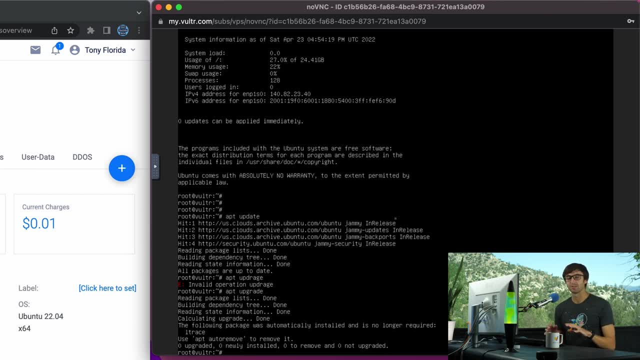 up to date. Now what we are going to do is use the apt package manager to install a web server for our VPS, and we're going to install the nginx web server. So to install a package in general, you do apt install and then the package name, which in this case is nginx n-g-i-n-x, hit enter and that's. 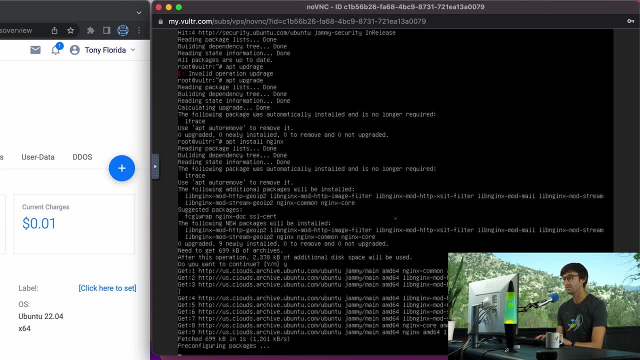 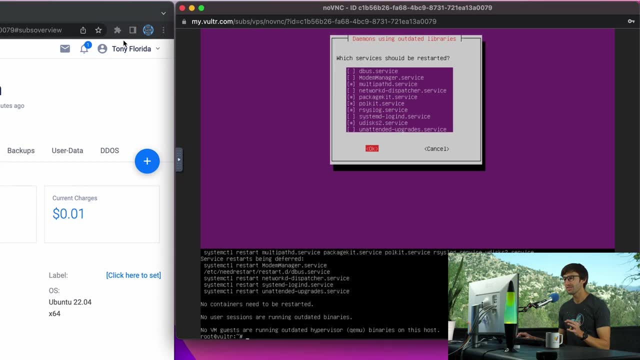 going to take about 2000 kilobytes of additional disk space. And if you get this prompt here, just hit the tab key and enter Okay, now that our nginx web server is installed, let's see if we can go to our website in a web browser. So let's copy our IP address. 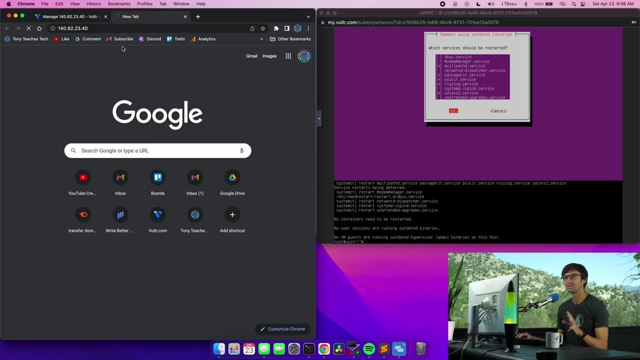 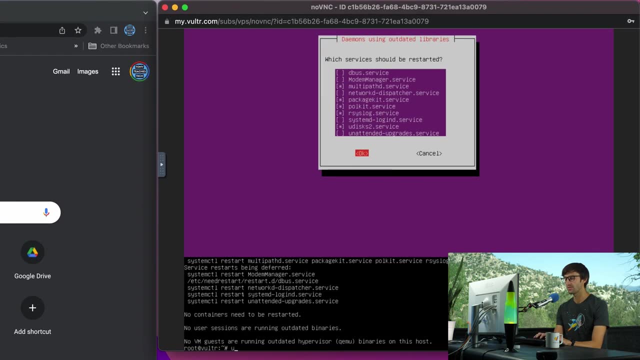 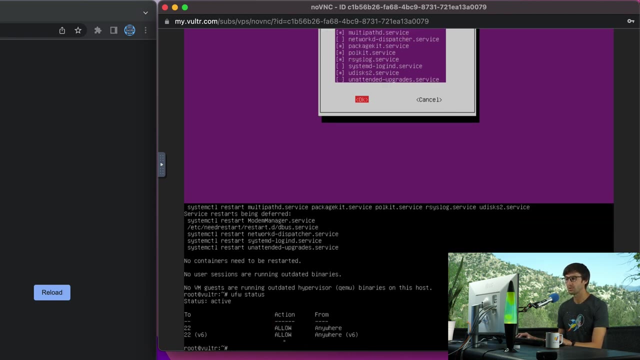 paste it in see if we get anything loading. and it doesn't look like it, It's just hanging here right now. The reason for that is because there is, by default, a firewall running. So if we do ufw, which is the ubuntu firewall status, it's only allowing connections from port 22, which is the 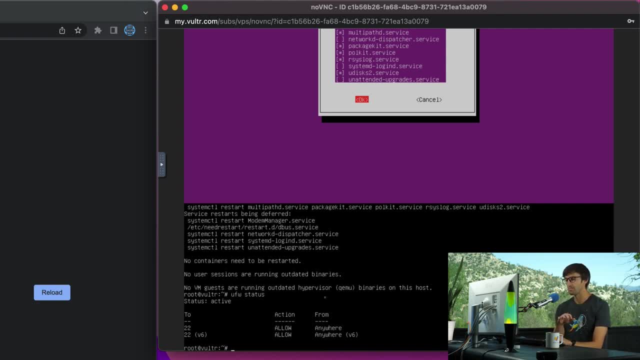 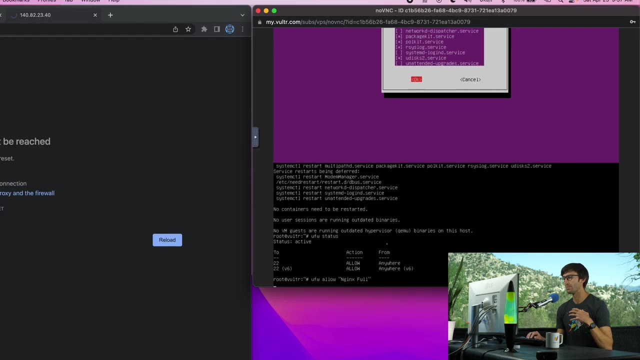 ssh port. So, in order to allow http ports or https ports, we can type something like this: ufw- allow. and then in quotes, double quotes, nginx full. And this is just a shorthand way to open up the those ports associated with that, And you can see immediately when we did that. 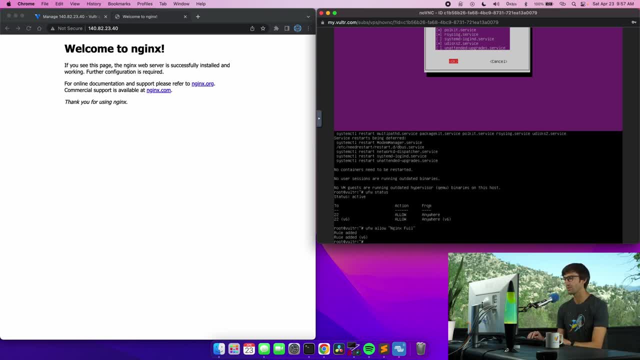 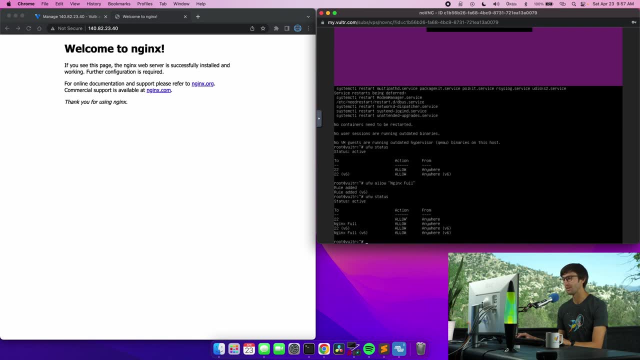 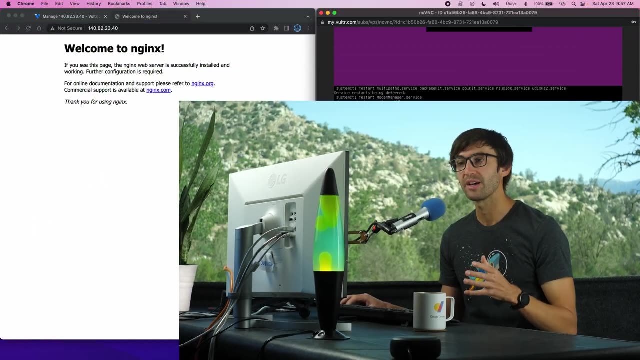 we see our nginx default landing page right here. So now if we do a ufw status, you'll see that we are allowing nginx ports open. they're allowed from anywhere. So whether you're new to hosting a website or not, I'm going to give you some basic overview. So this is actually html. there is a file. 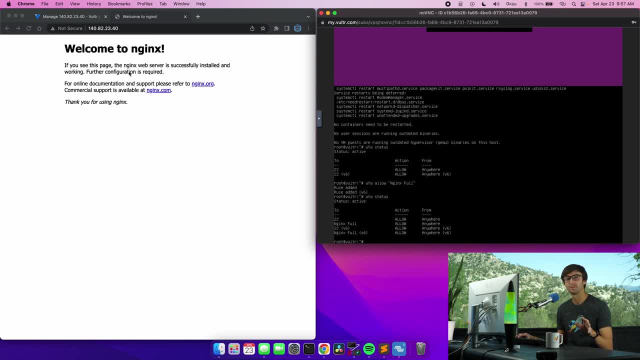 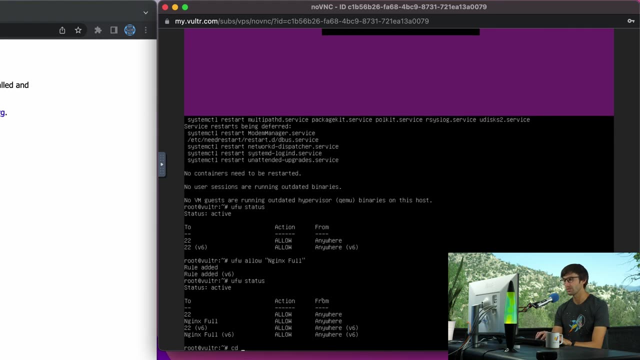 in the system an html file that we can modify to make our own web page, And that file, by default for dbn and a lot of Linux systems, is located at var- wwwhtml. So we can use the cd command to change our directory to that location. So cd slash, var slash, www slash, html, and in here we can use the. 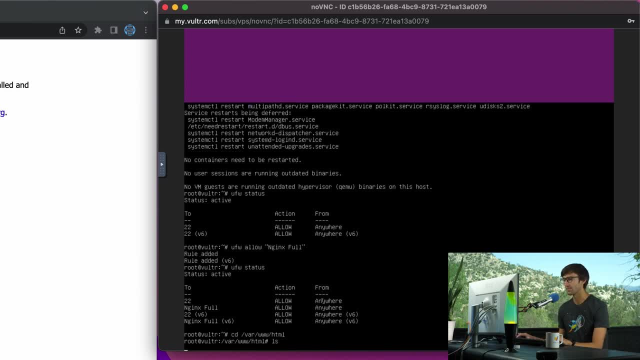 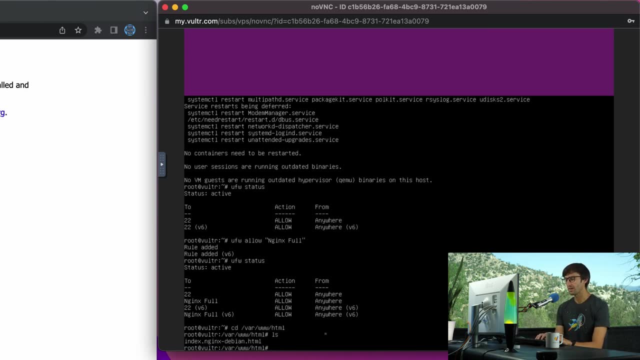 ls command to list out the contents of this directory. You'll see that we have an indexnginx-dbnhtml file, So let's open that up with a text editor. I think the most user-friendly text editor is nano, even though I like to use vim, but let's open it up. 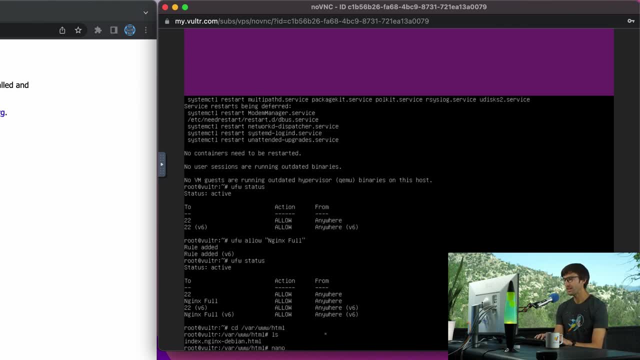 with nano, n-a-n-o and then the name of that file, So index. and what's cool about unix operating systems is that you can start typing a file and, as long as that's the unique, the only file in that folder that has those file names. So that way you can start typing a file and, as long as that's the unique, the only file in that folder that has those. 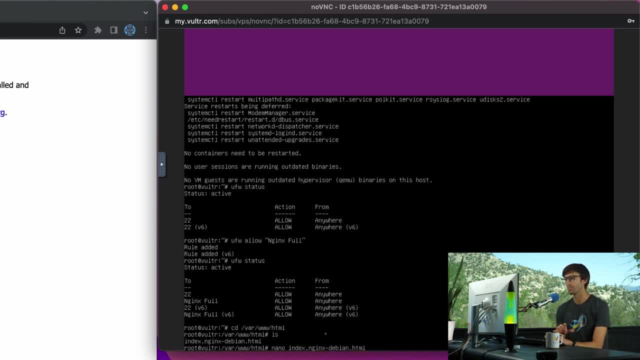 characters that you've typed, you can hit the tab key and it will auto complete that name, so you don't have to type out everything. So, basically, what this is saying is: let's edit this file with this text editor. So hit enter and now we have the contents, the html contents of this page. 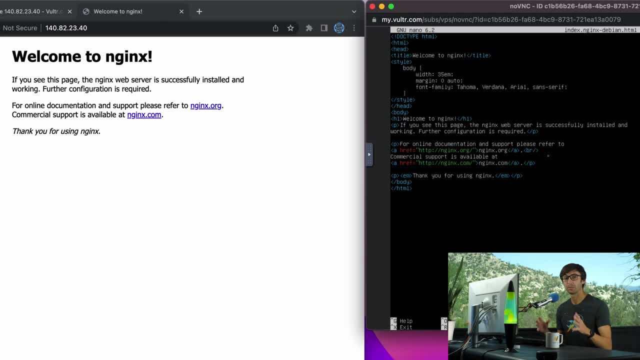 on the left. here. you can see them on the right. Now, what I'm going to do is actually modify this file to be a custom website for myself. I'm going to use it as a template, but feel free to do something else on your own. play around with html. 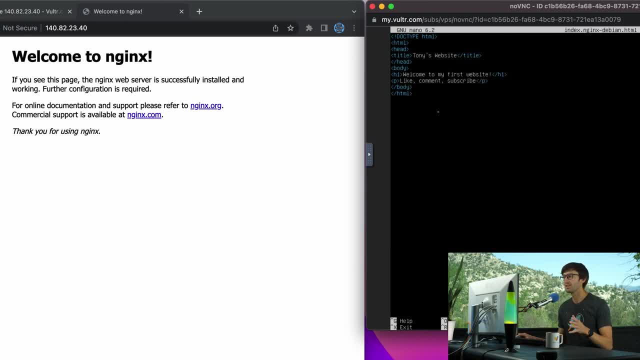 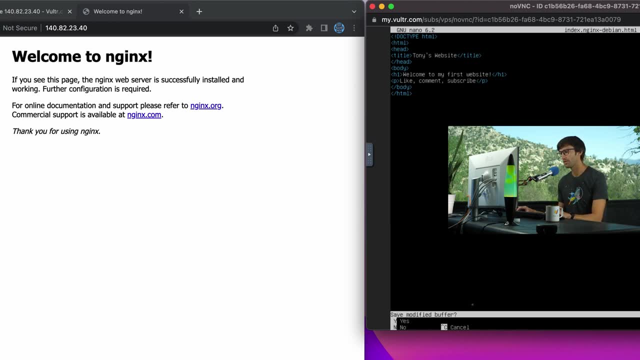 But yeah, this is what I'm going to do. Okay, there we go. when you're satisfied with your changes, you can save the file by typing ctrl x and it's going to say save modified buffer. You can type y for yes and then hit enter to get out of there. Now we are back to our terminal window and those